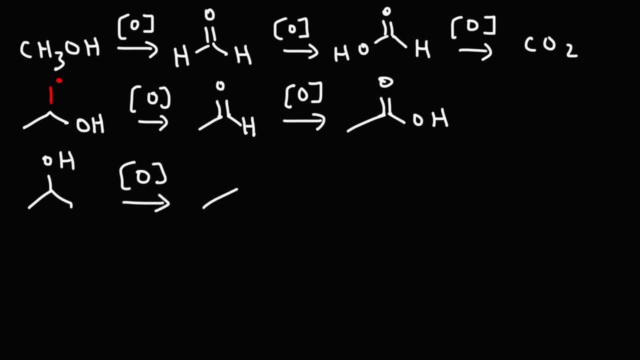 this is going to stop at the ketone level upon oxidation And tertiary alcohols? they're resistant to oxidation, So for the most part it's going to be no reaction, Unless, of course, you have a reaction that's capable of breaking carbon-carbon bonds. 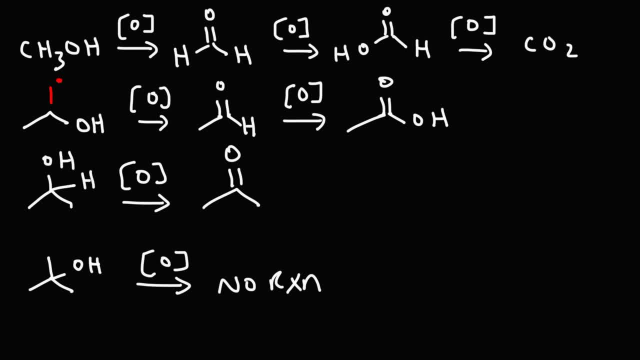 Now, one of the reasons why tertiary alcohols are resistant to oxidation is because they're resistant to oxidation. So if you have a tertiary alcohol, you're going to have a reaction that's capable of breaking carbon-carbon bonds. They don't have this alpha hydrogen that's present in primary and secondary alcohols. 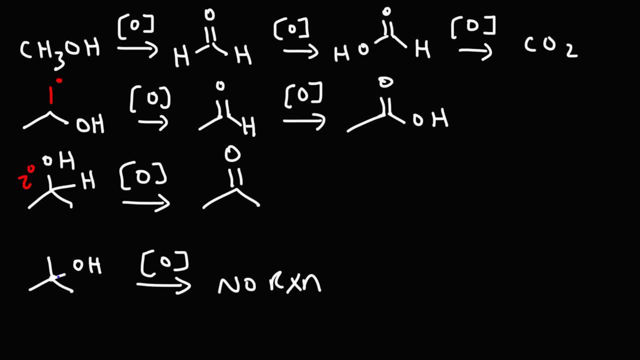 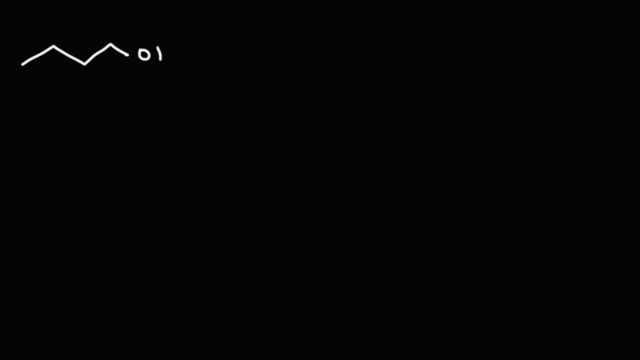 This carbon has no hydrogens on it, So that's one reason why tertiary alcohols are resistant to oxidation. Now let's go over some reagents that you want to be familiar with. Let's say we have one butanol and we want to react it with PCC. 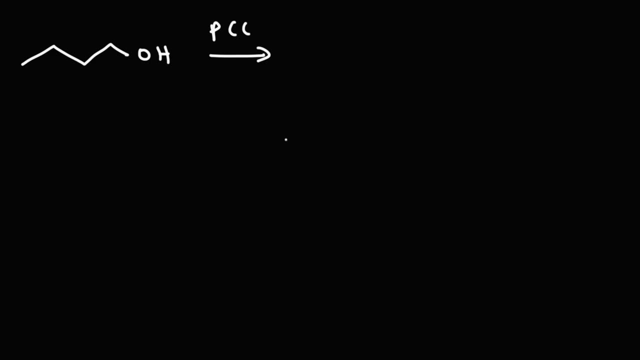 PCC will react to oxidation. PCC is pyridinium chlorochromate. When you see PCC, it looks like this: So you have pyridine. Pyridine is basically a benzene ring with a nitrogen inside of it. You also have hydrochloric acid and chromium oxide or chromium trioxide. So 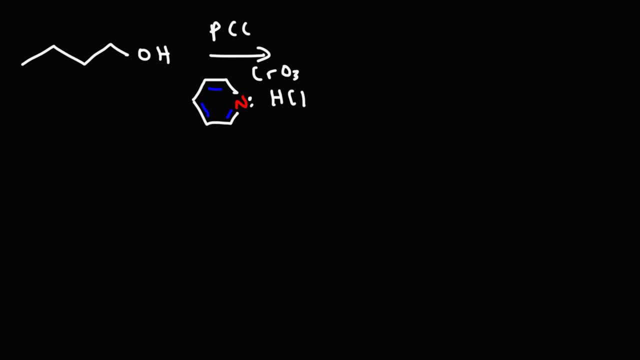 that complex makes up PCC, pyridinium chlorochromate. Now PCC is a mild oxidizing agent. It'll convert a primary alcohol to an aldehyde. If you were to use sodium dichromate Na2Cr2O7 under acidic conditions, this is. 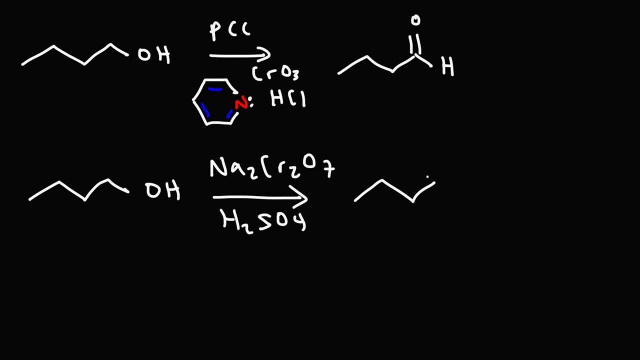 a strong oxidizing agent. It'll convert the primary alcohol into a carboxylic acid. In other words, it'll take it all the way If you were to react methanol with sodium dichromate, Na2Cr2O7,. this is a strong oxidizing agent. In other words, it'll take it all the way If you were to react methanol with. 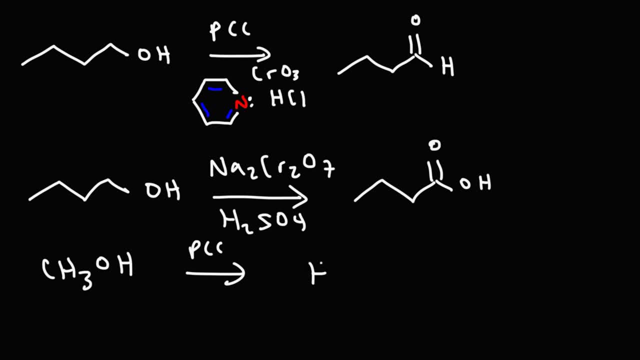 PCC? PCC will stop at the aldehyde level, so you'll get formaldehyde. But if you were to react methanol with sodium dichromate, Na2Cr2O7, or chromic acid Na2Cr2O7 under acidic conditions? 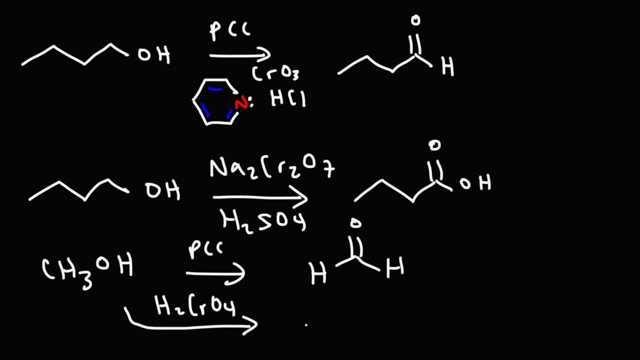 these are strong oxidizing agents. It'll convert methanol all the way to Cl2O7.. It will fully oxidize it. So if you see, chromic acid- Na2Cr2O7,, sodium dichromate, Na2Cr2O7,. 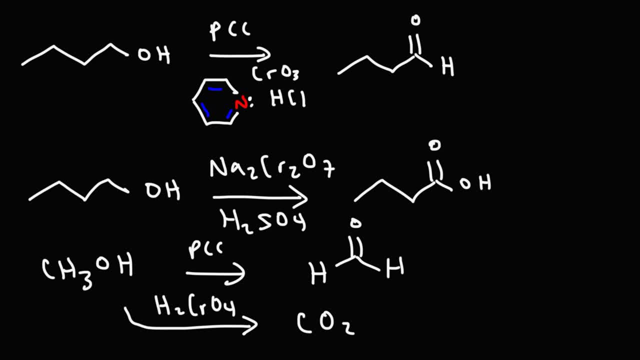 in acliconiodine, creatures in your bio Grande, morbid gene, coronary76, пес которых. Those are strong oxidizing agents. under acidic conditions, Pyridine with HCl. you no longer have a strong acid. What's going to happen here is this: nitrogen will grab the proton. 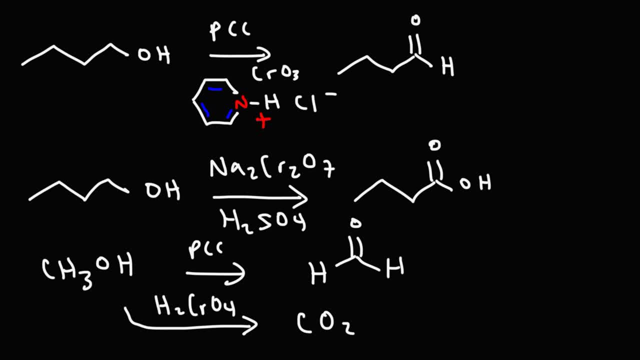 And so you now have a weak acid instead of a strong acid. So even though you have chromium in PCC, it's not under strongly acidic conditions. This is more of a weak acid when you combine pyridine and HCl, So the pH, the concentration of the acid, it greatly affects the oxidizing strength of chromium. 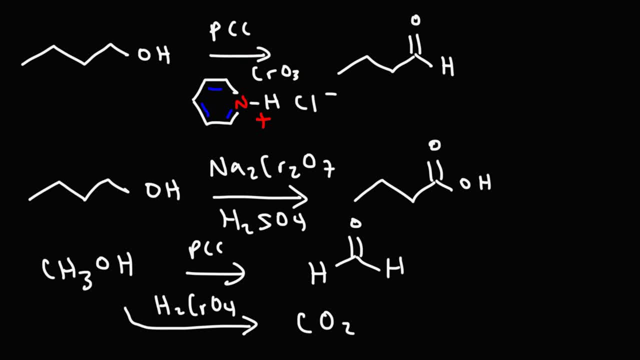 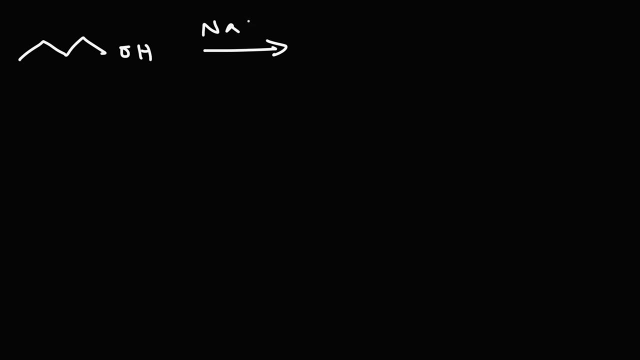 Now there are some other reagents that you want to be familiar with. If you use sodium hypochlorite with a weak acid like acetic acid at low temperature, this too works as a mild oxidizing agent. It'll convert the primary alcohol into an aldehyde. 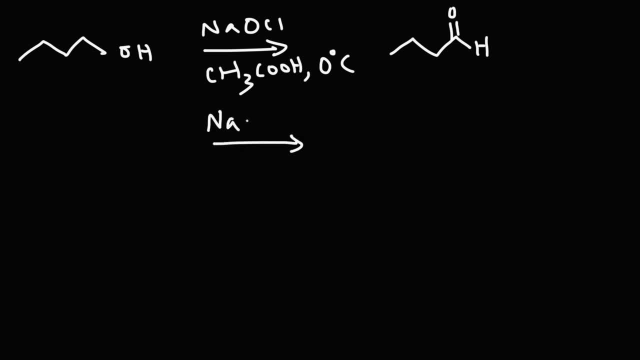 Another similar reaction is using sodium hypochlorite with a reagent called TEMPO. Like PCC, it's a mild oxidizing agent. TEMPO is a very stable free radical species. You have a nitrogen in a sodium hypochlorite. 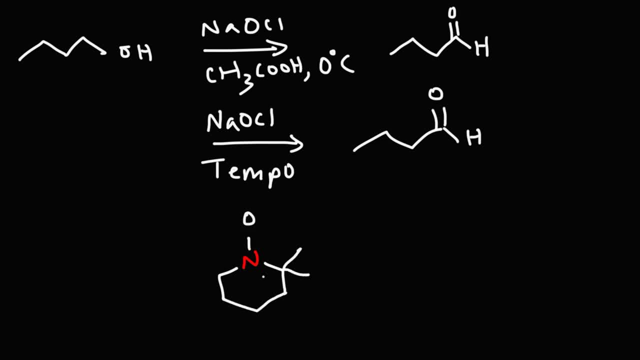 It's a 6-membered ring attached to an oxygen. Now, this oxygen is a radical. It has an unpaired number of electrons, But with sodium hypochlorite it works as a mild oxidizing agent. Now, another reagent that you want to be familiar with is this particular reaction called 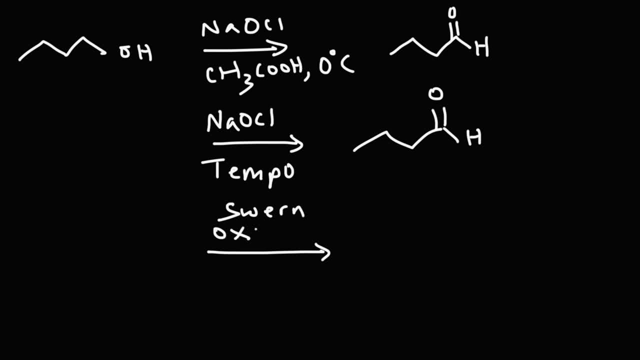 the Swerin oxidation. The Swerin oxidation uses reagents like DMSO, dimethyl sulfoxide, oxalyl chloride, triethyl anine and dichloromethane. This, too will convert a primary alcohol into an aldehyde. 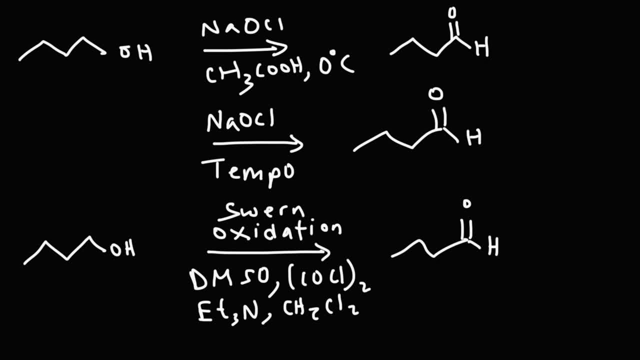 So it's a mild oxidizing agent. Now, if we were to take 1-butanol and react it with potassium permanganate under acidic conditions, this is a very strong oxidizing agent. It's going to oxidize it all the way. 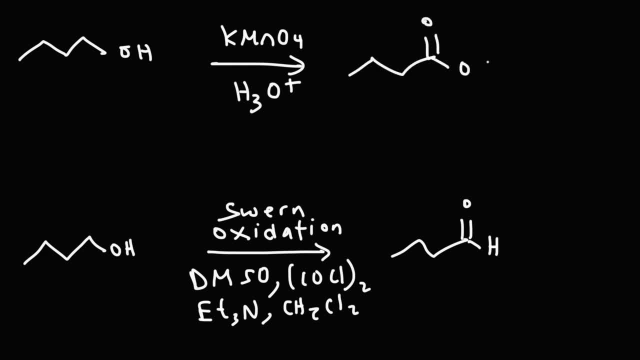 In this case for a primary alcohol. it's going to oxidize it to a carboxylic acid. Now there's some other reagents that you want to be familiar with, like the Jones reagent, the Collins reagent. Those are also oxidizing agents. 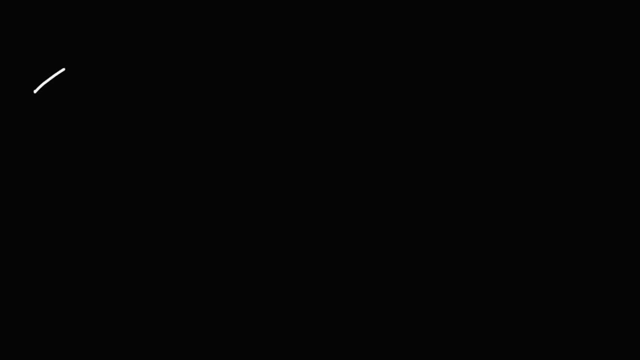 Now let's talk about the mechanism of the oxidation. Let me say that again, The oxidation reaction of: We're going to use 2-propanol Sodium hypochlorite With acetic acid, So the hypochlorite ion, it's a base. 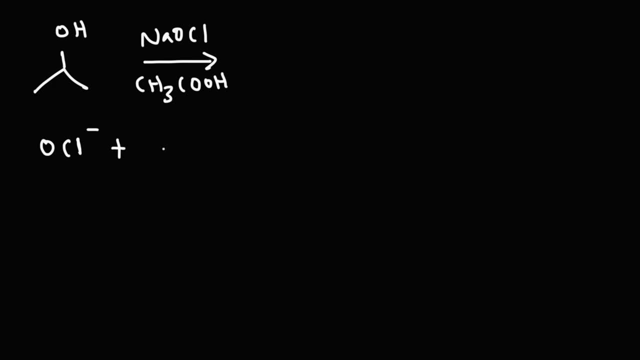 It's not a weak base. It's not very You wouldn't classify it as a strong base, but it's a significant base. When you react it with acid, it's going to convert into HOCl, which is a weak acid. 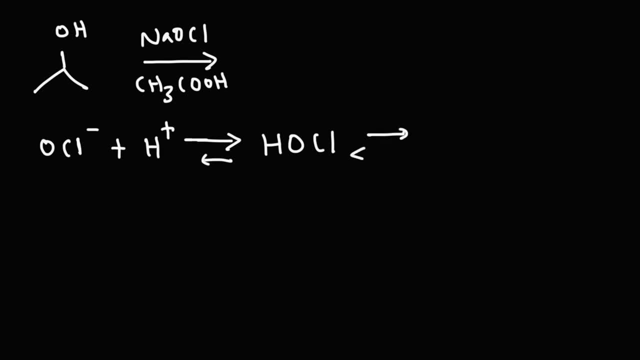 And upon reacting with additional acid, it could turn into this H2OCl+. Now notice the size of the arrow. The majority of OCl will be in this form. A very small amount will be in this form, because that form is not very stable. 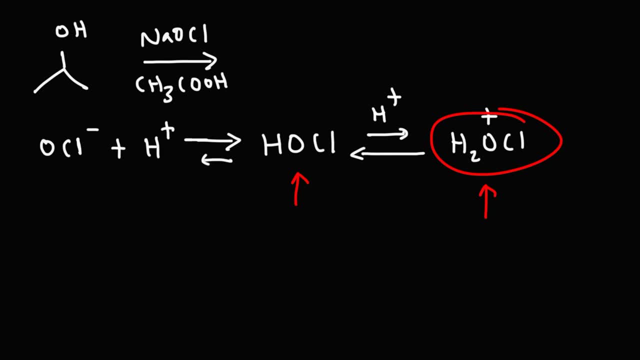 but this is going to be the reactive intermediate that we're going to focus on this reaction. So HOCl- hypochlorous acid- is a weak acid, but this is a strong acid. So here is H2OCl+. The oxygen is going to have a positive formal charge. 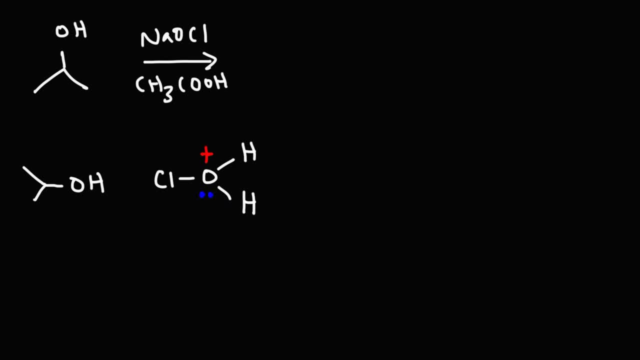 because it has three bonds in a lone pair. Now let's talk about the oxygen-chlorine bond. Which of these two atoms, would you say, is more electronegative? Chlorine or oxygen Chlorine, Chlorine, Chlorine. 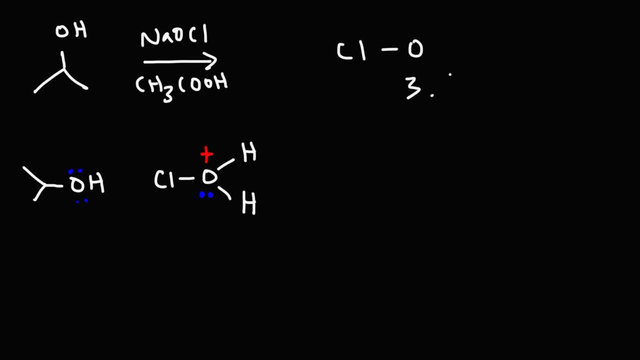 According to the Pauline scale of electronegativity, oxygen has an EM value of 3.5.. For chlorine, its electronegativity value is 3.0.. So oxygen is more electronegative than chlorine. Therefore now, this is different from formal charge. 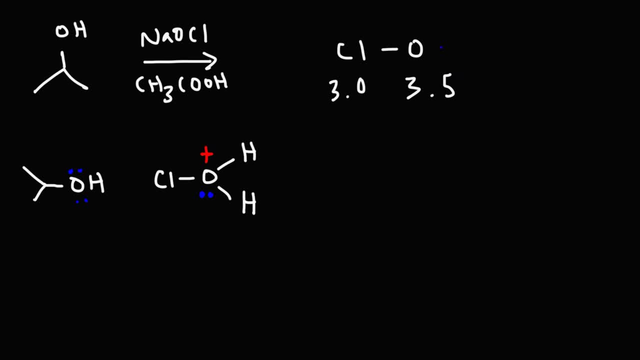 but in terms of partial charges, because oxygen is more electronegative, it's going to carry the partial negative charge. In the ClO bond, chlorine is going to bear the partial positive charge. So what this means is that this oxygen, which has a negative partial charge, 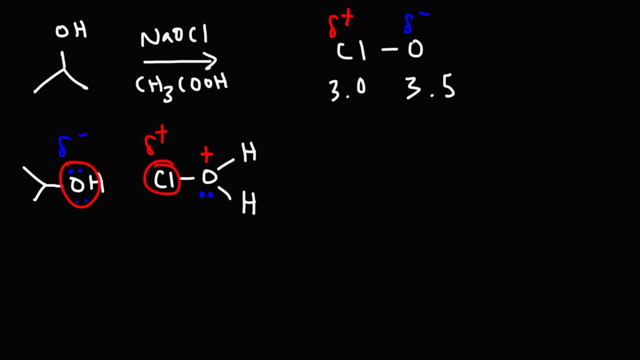 is going to be attracted to the chlorine atom, which has a positive partial charge. So we're going to have an SM2-like reaction, where the oxygen is going to attack the chlorine and we're going to kick out the leaving group, the leaving group being water. 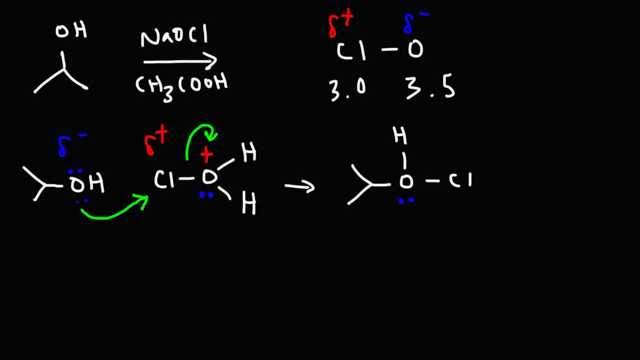 So this oxygen has three bonds now, so it's going to have a positive charge. and water was removed. Water is a good leaving group Now we could use water, but we're not going to use water, So we're going to have a positive charge. 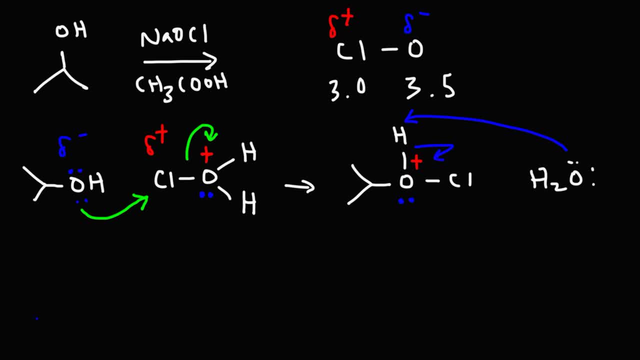 to remove this proton. Whenever oxygen has three bonds and a positive formal charge, any protons on it are relatively acidic. So now we have this reagent or this compound. Now, in order for oxidation to occur, we need an elimination. 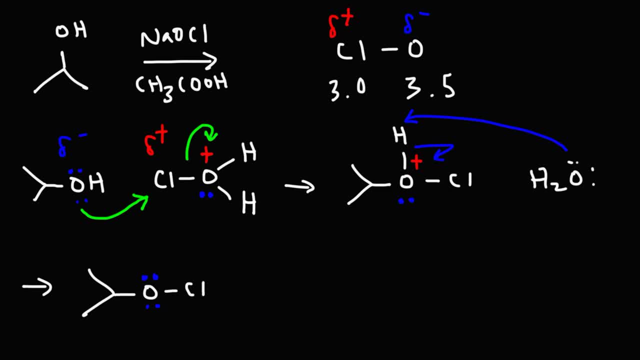 we need an elimination reaction. This is not like the E2 elimination reaction, where we would remove the beta proton. In this case we're going to remove an alpha proton. So just to compare, here's a typical E2 reaction. Bromine is the leaving group. 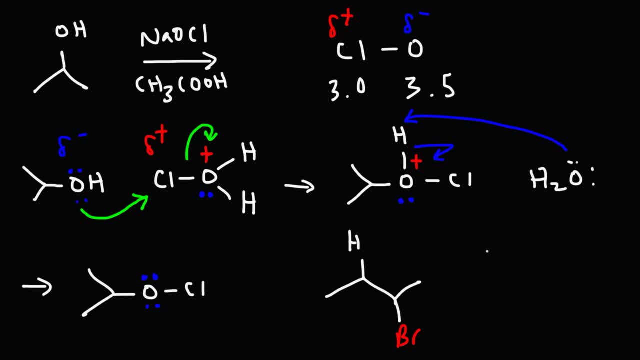 and hydrogen is the proton that we need to remove. So this is the carbon of interest, This proton here that is on the same carbon as the leaving group, that is the alpha proton. Adjacent to it is the beta proton. So in an E2 reaction, 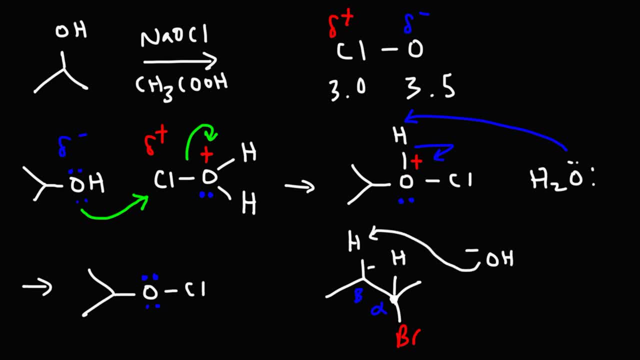 where we have a strong base, it removes the beta proton, not the alpha proton, And this is how we get an alkene. But for an oxidation reaction, the base is not going to remove the beta proton, It's going to remove the alpha proton. 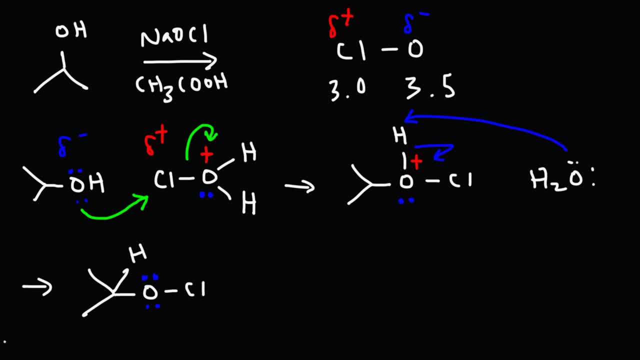 The alpha proton is on the same carbon as the leaving group. So we could use water as a base or we could use acetate. Let's use acetate. So acetate is going to act as a weak base. It's going to go for the alpha proton. 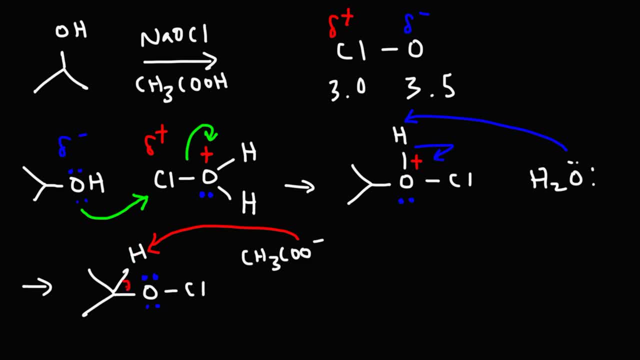 The carbon-hydrogen bond will break. Those electrons will be used to form this pi bond. So we're not getting an alkene, but we're getting a double bond like an E2 reaction, And then the leaving group, the chlorine, is going to leave. 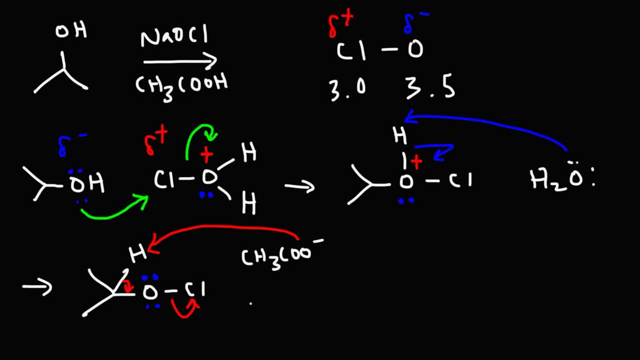 So that is an example of an alpha elimination reaction. The end result is that we get a ketone. So that's the general idea of the mechanism of an oxidation reaction. You need a base to remove the alpha proton, which will allow us to form a pi bond. 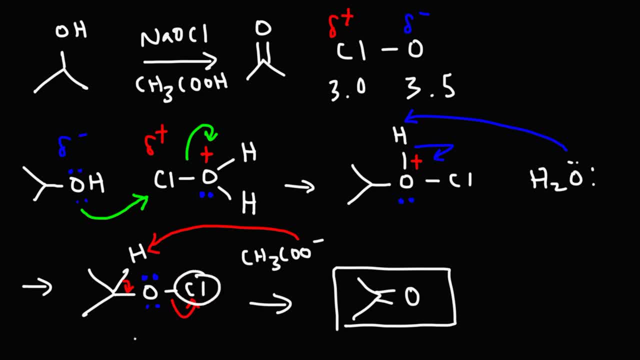 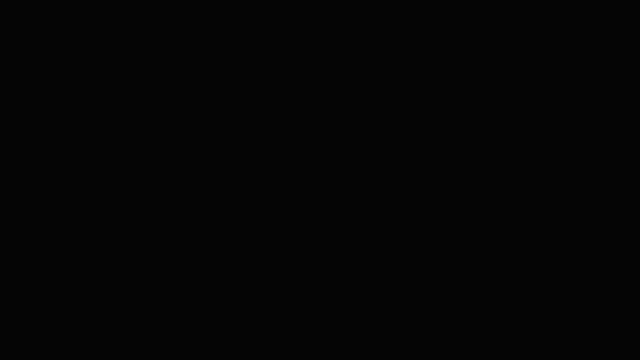 And there needs to be a leaving group on this oxygen that we can kick out. Once we have all of that, we can oxidize the alcohol into an aldehyde or a ketone. Now here's a question for you. Let's consider phenol. 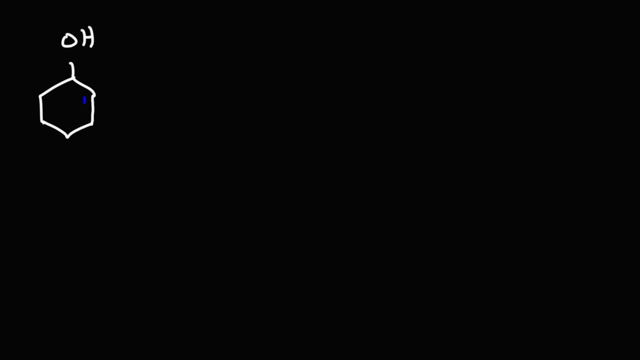 Can phenol be oxidized? What would you say If we were to react phenol with sodium dichromate and sulfuric acid? can this be oxidized? And what if we were to react this with tert-butanol? Let's use chromic acid. 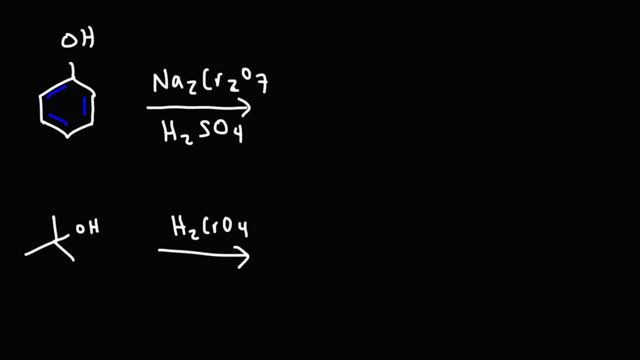 What would we say? Tertiary alcohols, for the most part, are unreactive towards oxidation reactions. So for our practical purposes we could say no reaction for this process And, as we could see, there's no alpha hydrogens on this carbon. 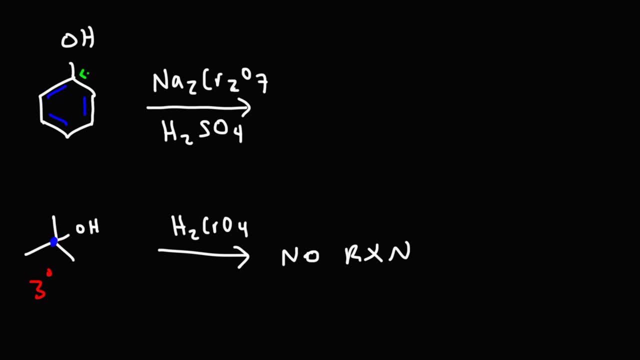 Now you might apply the same approach to phenol, saying that, hey, there's no alpha hydrogens on this carbon, so it would appear as if phenol will not be oxidized. However, the hydroxyl group is attached to a benzene ring. 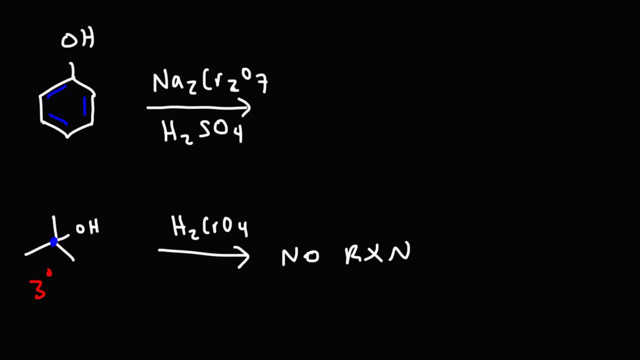 So you have free-flowing pi electrons here, And it turns out that phenol can be oxidized into this compound, benzoquinone. So even though phenol doesn't have any alpha hydrogens, it can be oxidized due to this aromatic ring. 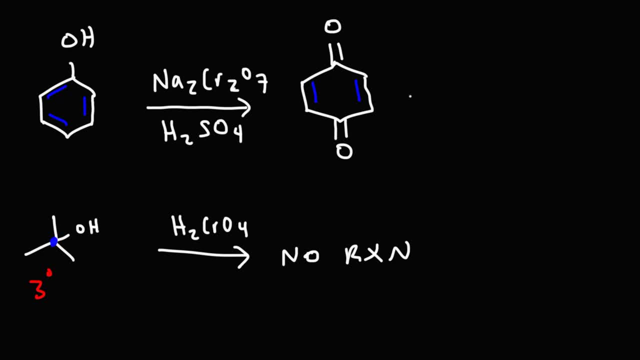 and those free-flowing electrons. Now benzoquinone can be reduced to hydroquinone. Hydroquinone looks like phenol, but you have two hydroxyl groups as opposed to one. So you have two hydroxyl groups as opposed to one. 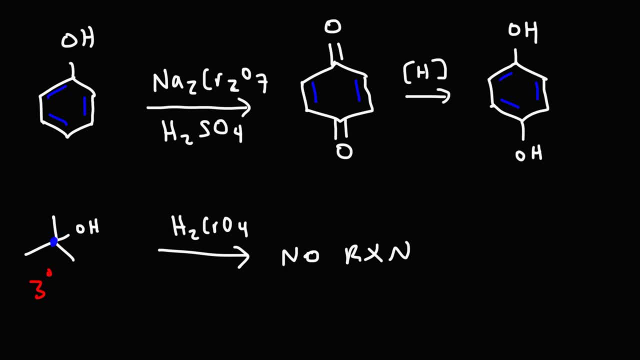 So make sure you're aware of that. Even though phenol doesn't have any alpha hydrogens on the carbon that bears the hydroxyl group, it can still be oxidized, So it's a different case than a typical tertiary alcohol. But that's basically it for this video.